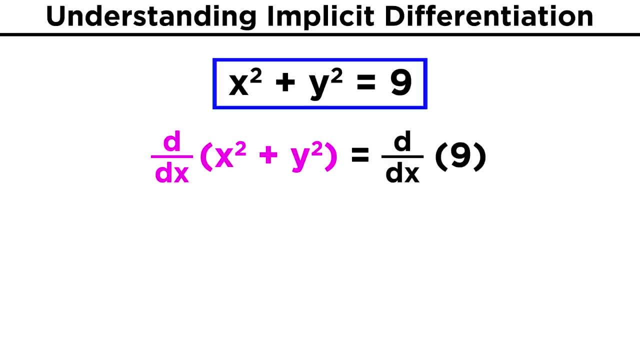 We know that the derivative of a sum is just the sum of derivatives, so we can change this to the derivative of x squared with respect to x, plus the derivative of y squared with respect to x. On the right, the derivative of any constant is zero, so that becomes zero. 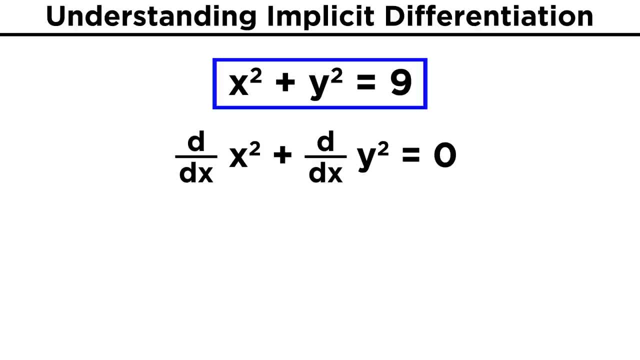 Now let's evaluate these terms. This is the part we have to really wrap our heads around. We are specifically treating y as a function operating on x, and we should therefore imagine f of x. anywhere we see y. So when we take the derivative of x squared with respect to x, it's just what we are. 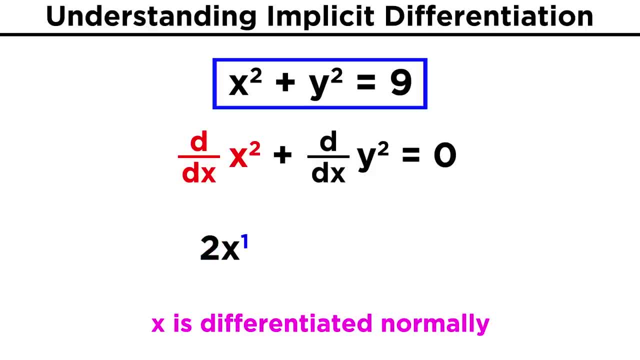 used to Two comes down here, the exponent becomes one and we get two x. But for y squared it's different, Because we are not taking the derivative with respect to y, it is still with respect to x, and again we are thinking of y as a function that depends on x. 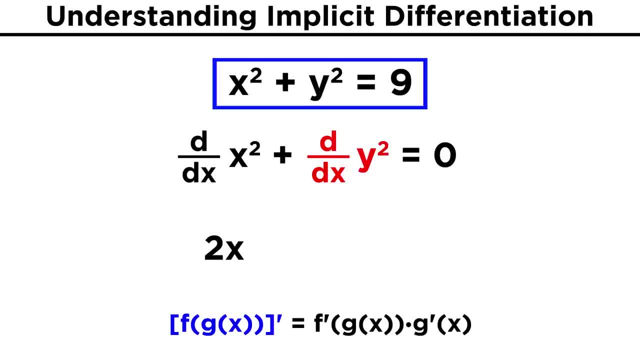 For that reason we have to use the chain rule. Remember that the derivative of a composite function is the derivative of the outer function times the derivative of the inner function, and we imagine this as f of x raised to the second power. So here we will take the derivative of y squared. 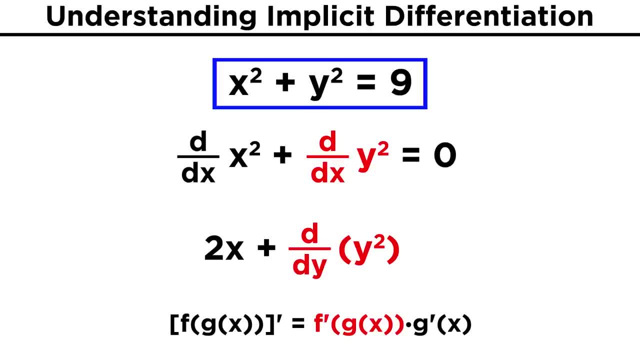 The derivative of y squared with respect to y, thinking of this exponent as the outer function operating on y, but then also imagining y as some other expression with x's in it. so we multiply by the derivative of y with respect to x, which is dy over dx. 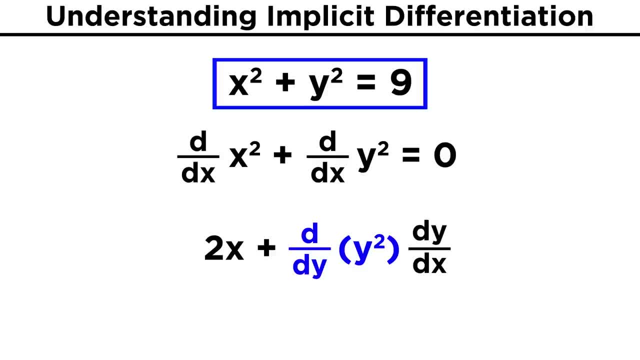 The derivative of y squared with respect to y is easy. that's just two y, as we would expect. Then we are left with dy over dx. We'll also just call y prime, and this is precisely what we are looking for. so let's. 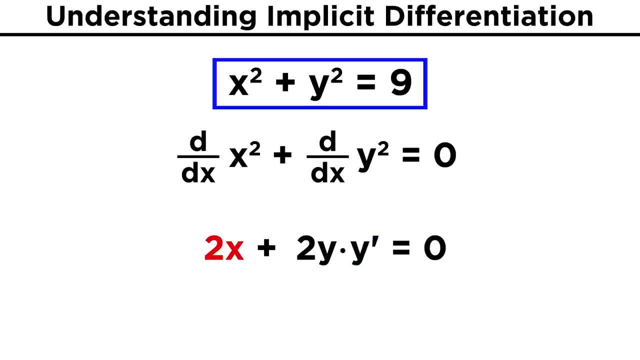 solve for it. Subtract two x from both sides, divide both sides by two y, and we are left with negative x over y. So this is y prime, or the derivative of the original function with respect to x. Here's a slightly trickier one. 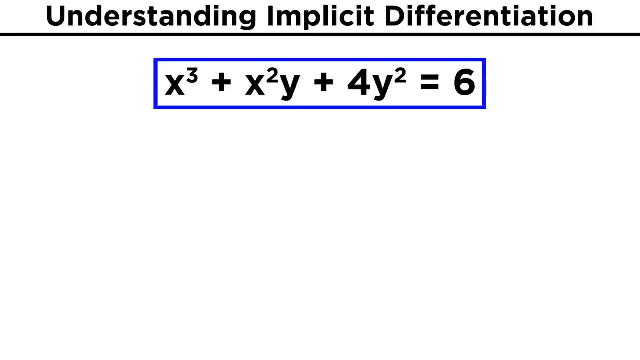 X cubed plus x squared y plus four y. So this is y prime or the derivative of the original function with respect to x. Here's a slightly trickier one: X cubed plus x squared y plus four, y squared, equals six. 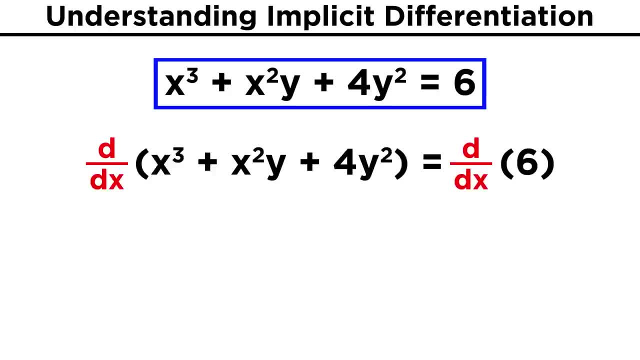 Again, we will take the derivative of everything with respect to x and we can treat each term in the sum separately. X cubed is easy. since there's no y, we just get three x squared, as we would expect. Now, for this second term, we have to use the product rule, since it's a product. 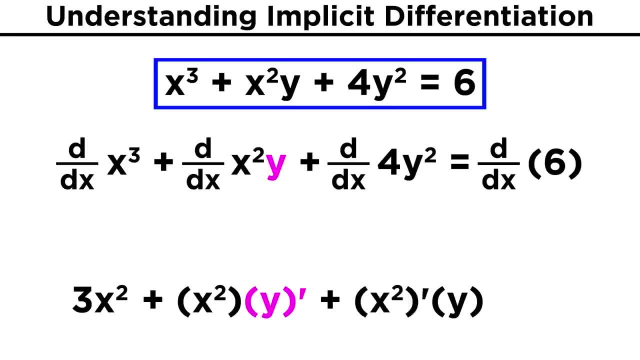 So let's write x squared times the derivative of y, plus the derivative of x squared times y. Now we evaluate these derivatives. The derivative of y will be y prime. Remember, y is a function and its derivative is some other function, which is what we are. 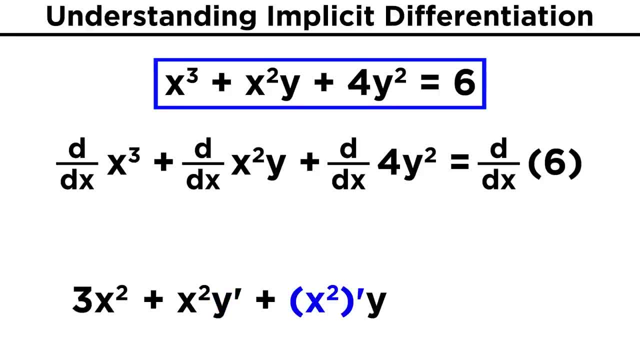 looking for. so we just write y prime. The derivative of x squared is two x. So we have x squared y prime plus two x y. And then we move on to the four y squared term. Here we need to use the chain rule. 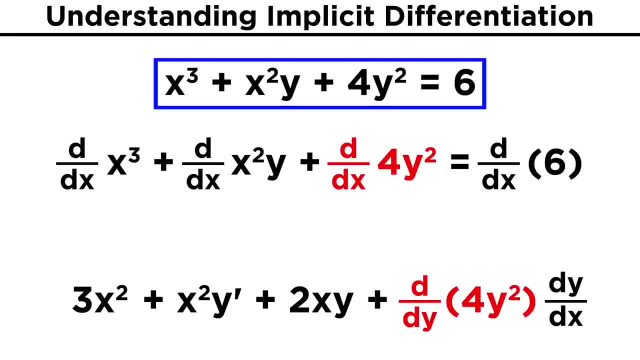 So we take the derivative with respect to y first, ignoring what's inside y, giving us eight y, But then we multiply by the derivative of y with respect to x, giving us y prime. So that will be eight y y prime And six becomes zero. 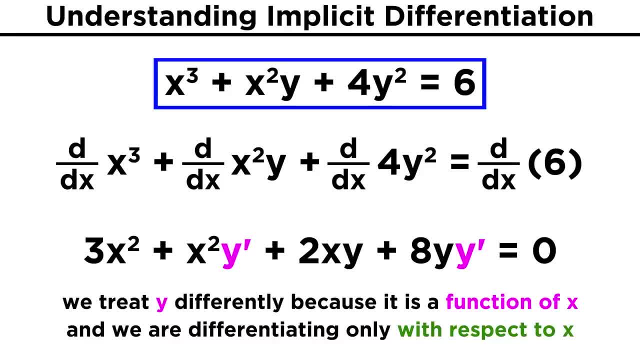 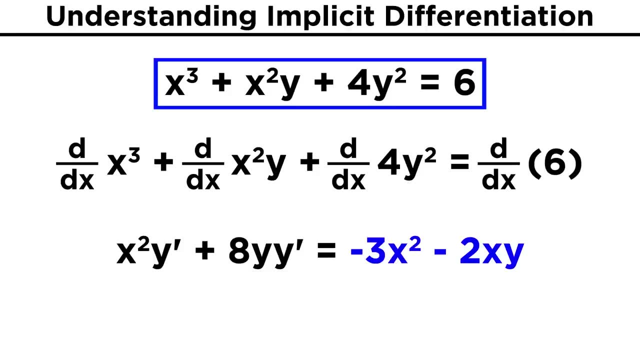 Remember, we do this extra stuff with y only because we are differentiating with respect to x and not y. Now let's bring all the terms without y prime in them to the other side. We do this so that we can then factor y prime out of these two terms. 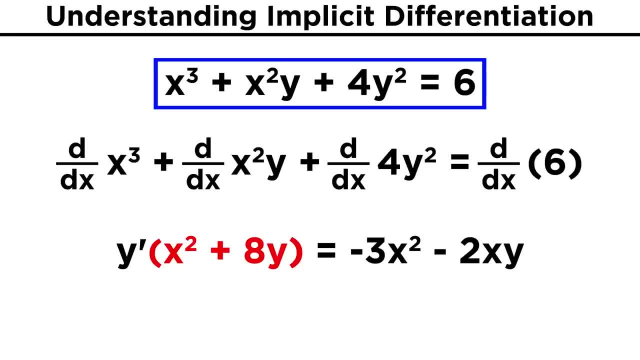 We do this so that we can then divide both sides by this parenthetical term, allowing us to solve for y prime, which is the point of all this. Then let's just factor a negative x out of the numerator for good measure, and we are. 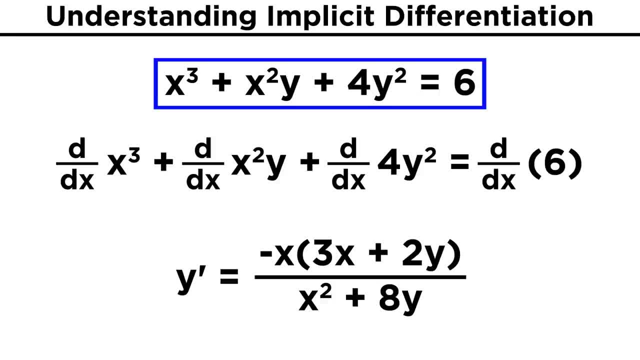 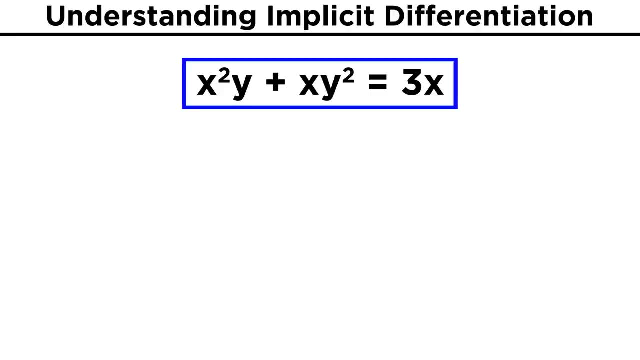 left with y prime equals negative x times the quantity three x plus two y divided by x squared plus eight y. Let's try another example of similar difficulty, just to make sure we have this: How about x squared y plus x? y squared equals three x, and again we want to differentiate. 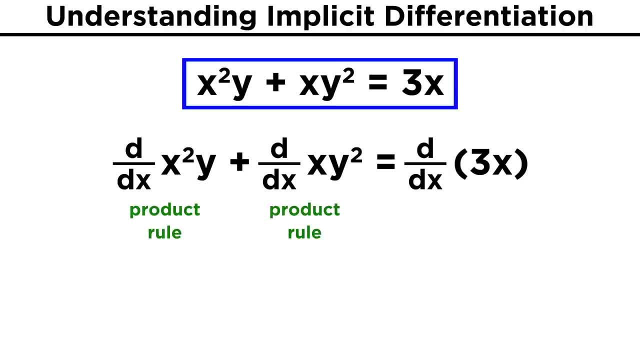 with respect to x. On the left We have two products, so we have to use the product rule for each of them. Taking the first one, we get x squared times the derivative of y, which is y prime. To that we add the derivative of x squared, or two x times y. 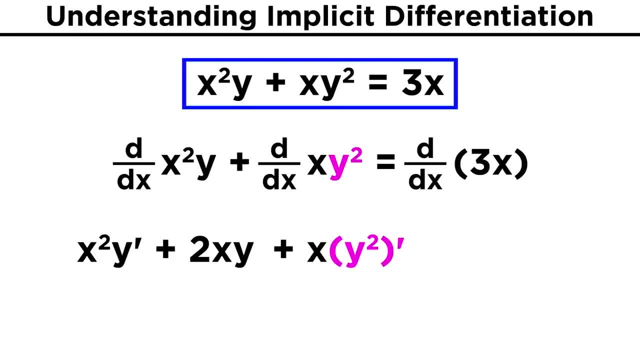 Now we do the other product, This will give us x times the derivative of y squared and once again, any time we take the derivative of the variable representing the function, we get x squared times the derivative of y squared. If we take the derivative of the function and there are other operations on that variable. 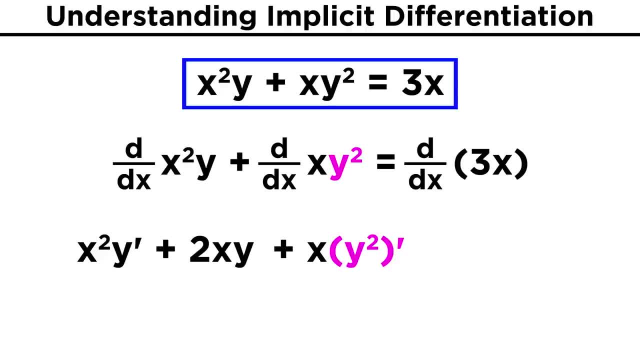 we must use the chain rule. So the derivative of y squared will be two y times y prime. Again, this makes sense if we imagine y as being some function full of x's. If that were inside parentheses and then squared, we already knew from learning the chain rule. 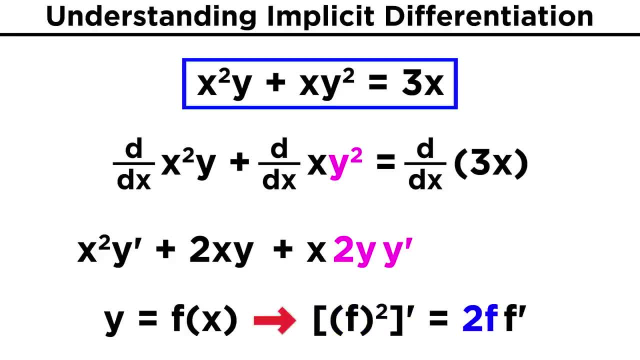 that the derivative of this would be two times what's inside the parentheses times the derivative of what's inside the parentheses. That's what we are doing here, just with y representing whatever might be in there. And then, to finish the product rule, we get the derivative of x, which is one times y. 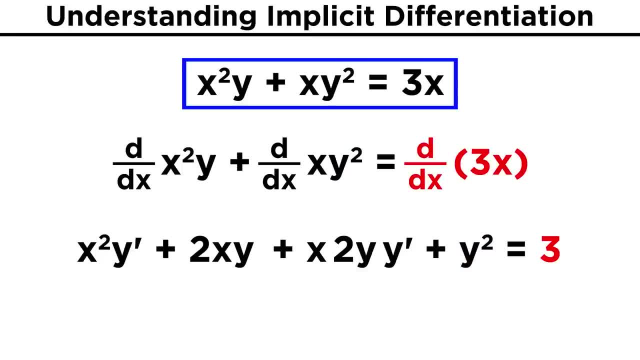 squared On the other side, three x becomes three Once again. let's keep any terms with y prime on this side and bring the other terms to the other side so that we can factor a y prime out of this sum. Once we have done that, we can then divide both sides by this whole parenthetical term. 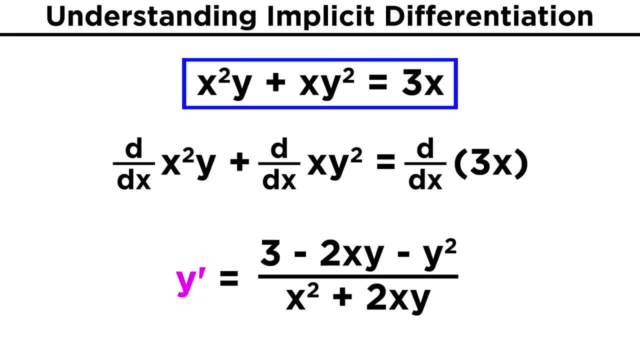 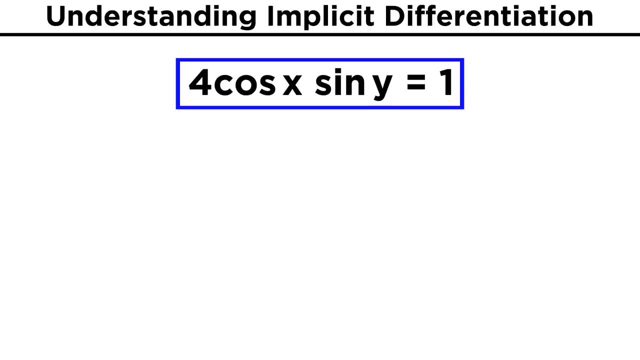 which allows us to solve for y prime. That gives us three minus two x, y minus y, squared all over x squared plus two xy. Let's do just one more. that looks a little different. How about four? cosine x, sine y equals one. 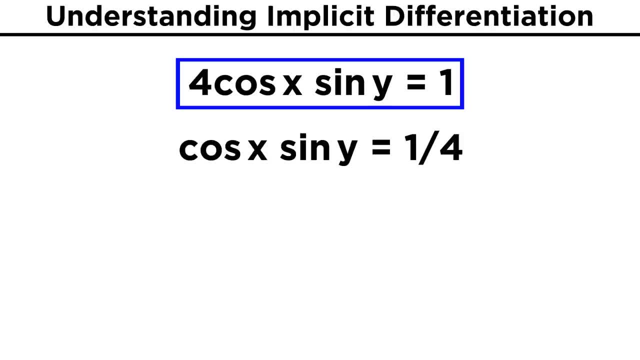 What do you think? Well, first let's divide both sides by four. That will make things a little easier, since one fourth will become zero anyway, and then we don't have to deal with the four. Now for the left side, we have a product, so let's use the product rule.